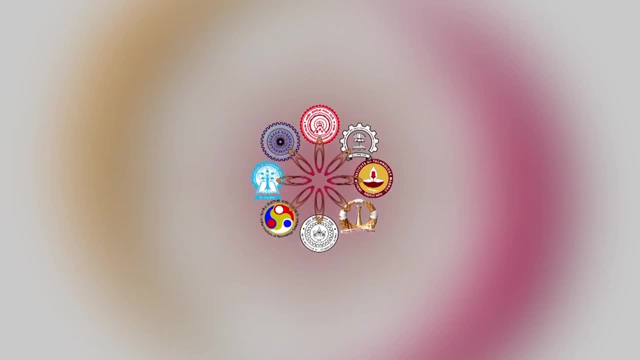 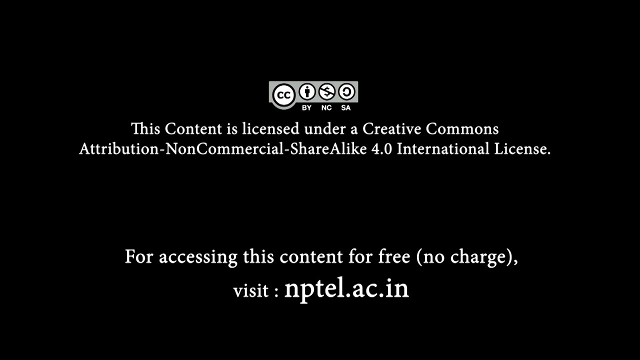 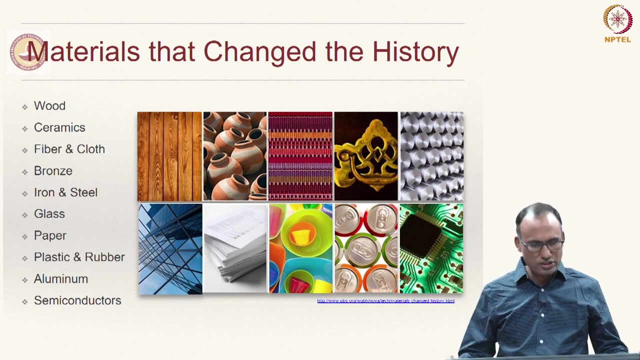 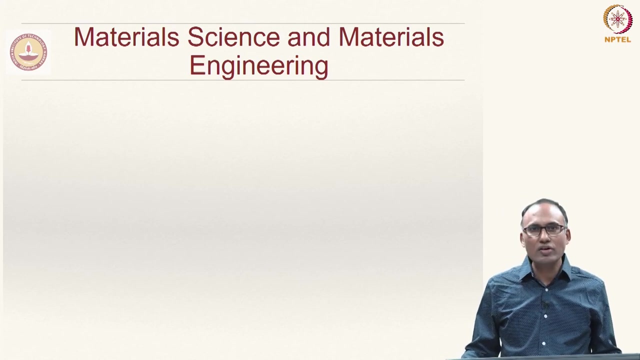 So far, we have looked at the materials that change the history. So we looked at wood, ceramics, fiber and cloth and so on. So now let us look at the concept of what do we mean by material science and what do we mean by materials engineering? or in other words, let 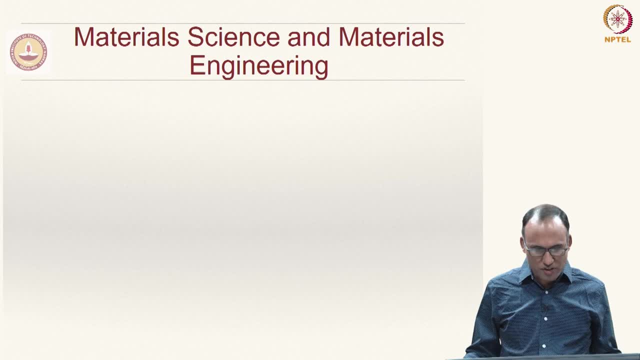 us see what is how these two fields of study have been classified. So the material science per se actually deals with the structure property correlations. So basically, what is the structure and what is the property that is obtained in the material through that structure? So material science deals with the structure property correlations. 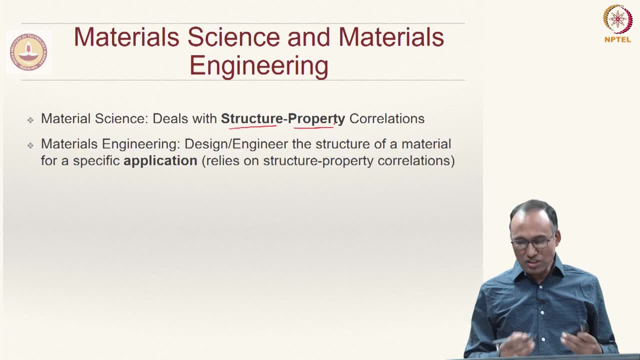 while materials engineering deals with designing or engineering of the structure of a material for specific application. So basically, it relies on structure property correlations and it takes from there and then tries to design structures or components for a material of a material for a specific application in mind. So what? 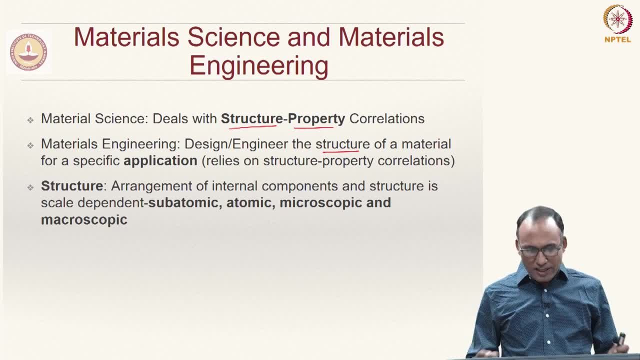 do we mean by structure? Structure is nothing but the arrangement of internal components, and it is actually scale dependent. So what do we mean by arrangement of internal components? What are the components that we are looking at? So, depending on the scale at which we are looking at, or depending on the resolution, 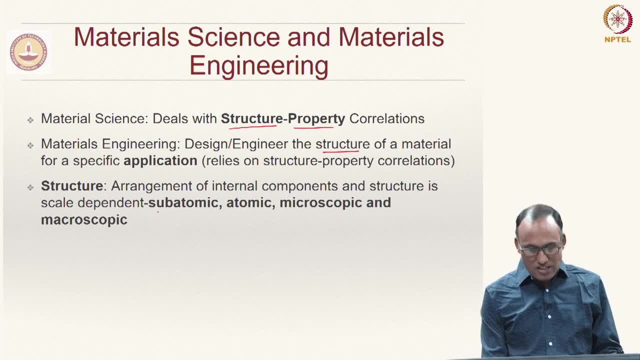 at which we are looking at. So what are the components that we are looking at? So, depending on the scale at which we are looking at, The structure can be, yes, subatomes structure, where- and we are actually looking at- All the electrons, protons and neutrons within atom are arranged, or an atom at a higher resolution. 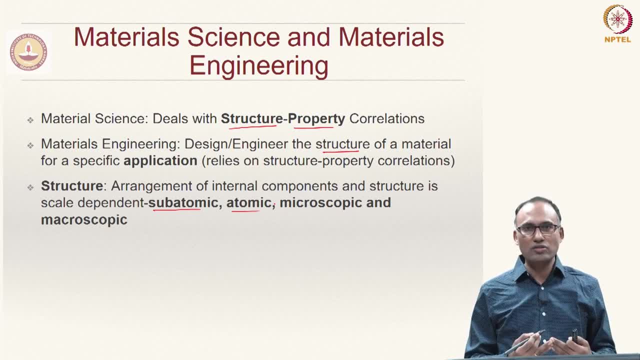 higher length scale. I want is the structure at a far slowly So the dimension. that means how the atoms are arranged in a given material, And later, at much higher length scale, You can have a microscopic structure where in how the according to tell the ch arm, is it not? do you know how the residence 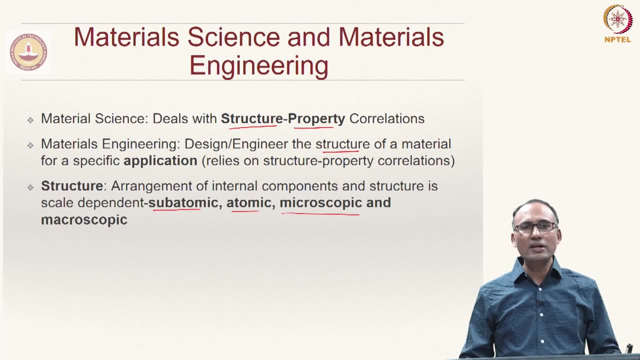 rari In termssol, sred, In terms waste, A green or and so on aren't arranged. So our next, And then finally the microscopic structure, meaning how the at the component level, how the structure is, how the system is looking like. 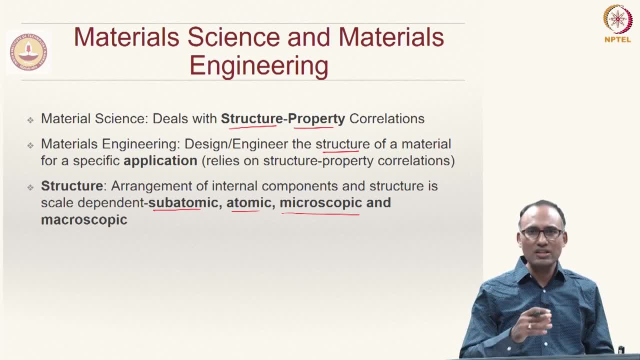 So the structure when we have, whenever we are talking about structure, it is actually a scale dependent phenomena. that means we should know at which resolution we are looking at right. So in order to get the information necessary for us, we need to choose the right resolution. 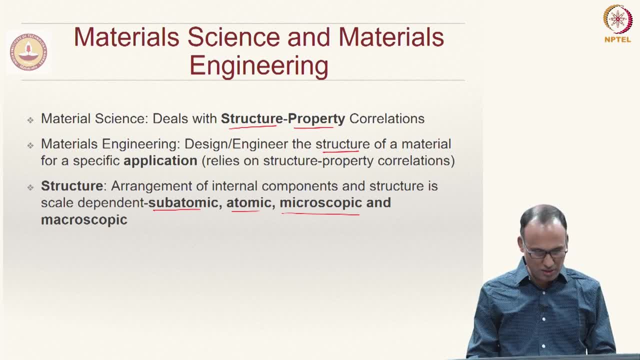 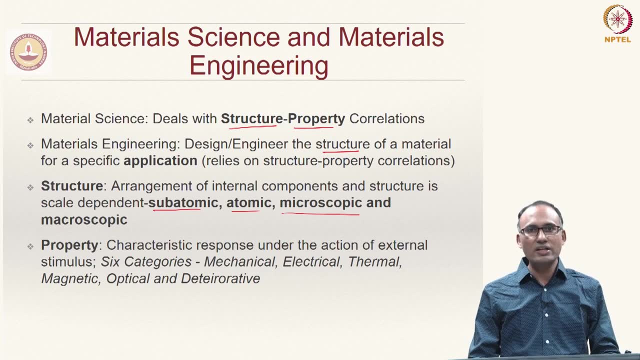 at which we need to look at in order to understand the structure. at that position, And when we say property- because the material science, as we have said it is, deals with- it- actually deals with structure, property correlation. So we have defined what is structure, but then what do we mean by property? 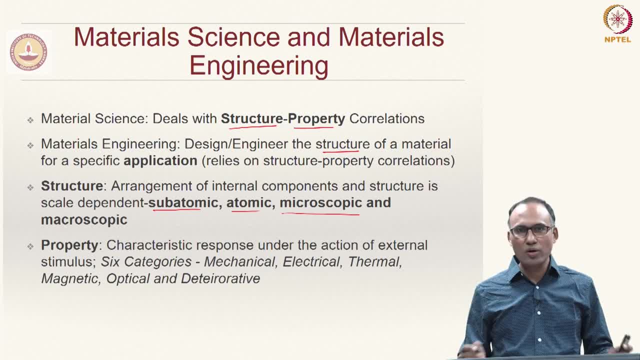 So property, by definition, is the characteristic response of any system under the action of some external stimulus. So if you give an external stimulus to a system, then the response of the characteristic response So offered by the system is called the property of the system. 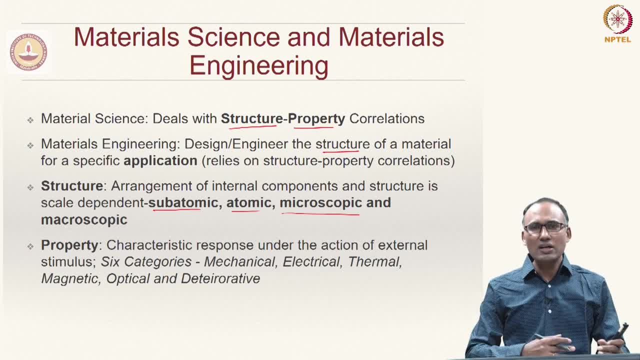 So what are the different kinds of external stimulus that one can apply? there are. we have primarily categorized them into 6 categories like mechanical, electrical, thermal, magnetic, optical and deteriorative properties. right So, mechanical means if you apply an external load, electrical means in an electric field. 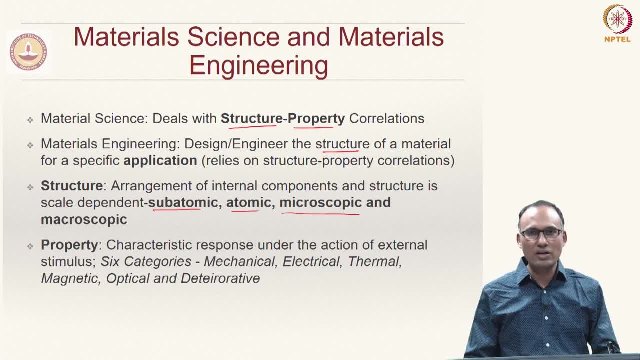 applied to a material and how the response- electrical response- of the material looks like When you are applying a mechanical load, how the deformation behavior that is the characteristic property right. So, for instance, elastic modulus is a property of the system that depends on the intratomic. 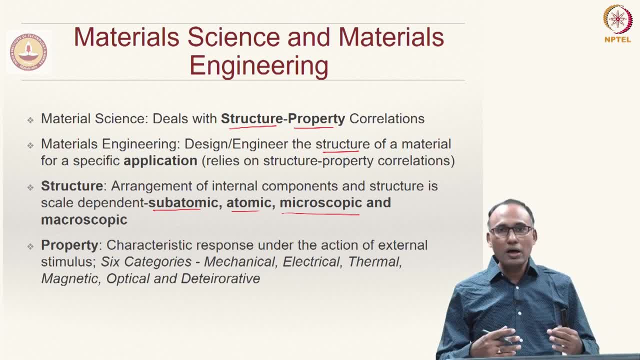 bonding in the material right. So you need to know the intratomic bonding, the how the intratomic bonding is existing in the particular material and that gives rise to the property called elastic modulus. Some other properties might require the information at higher length scale right. 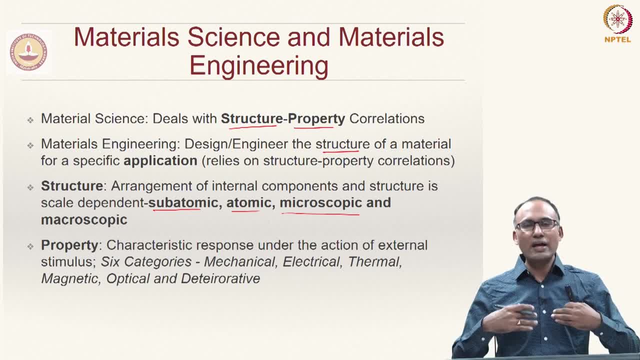 For instance, if you are talking about yield strength, then we are actually talking about dislocation motion, So that is at a much higher length scale than the individual bonds between the atoms and similarly thermal, magnetic and deteriorative. when we say deteriorative property, we are 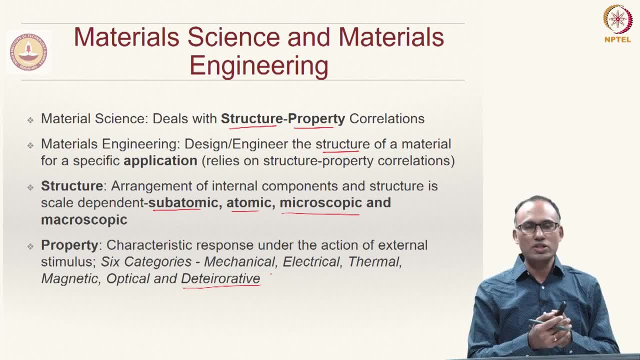 actually talking about, say, for instance, corrosion. So corrosion is a chemical phenomena. So that depends on the environment and depending upon the material that we are looking at. some of the materials in a particular environment might actually corrode faster compared to other materials, right? 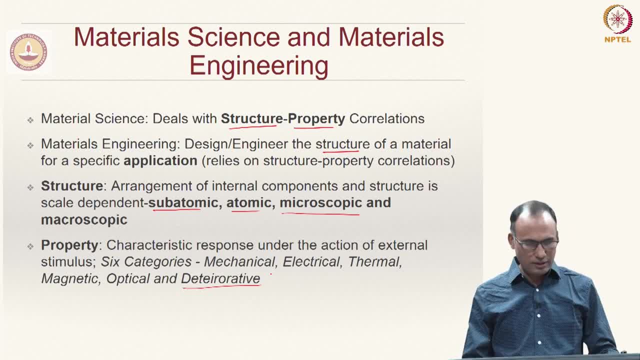 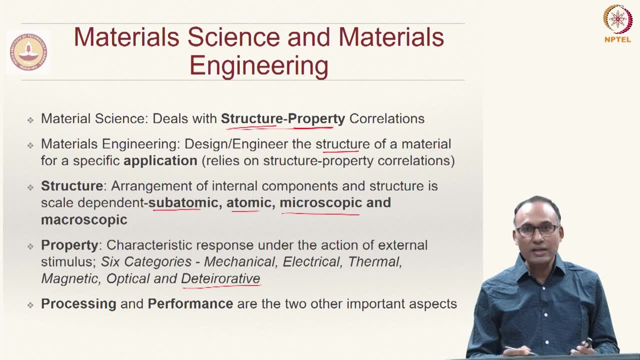 So that is also an important property of a material. So that is also an important property of a material. So that is also an important property of a material. And then, in addition to the structure and property which we have already introduced as the main objective of material science, there are two other important aspects to the 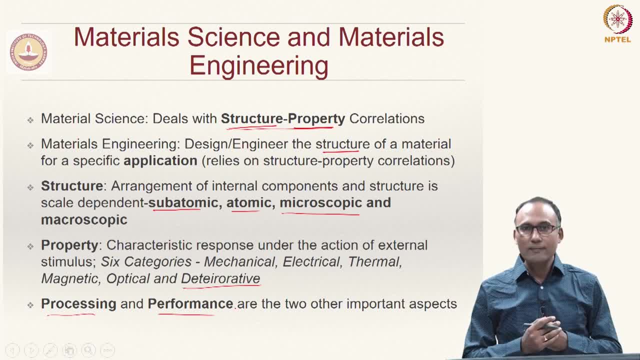 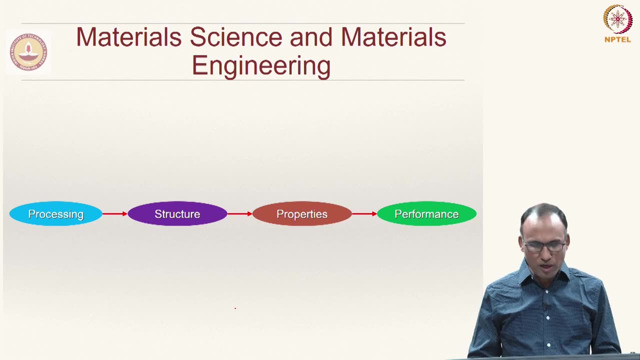 study of material science and engineering, that is, processing and performance, And these two aspects will actually connect this structure and property to give a broader understanding of these material science and engineering. So this diagram is popularly known as PSPP diagram in material science. 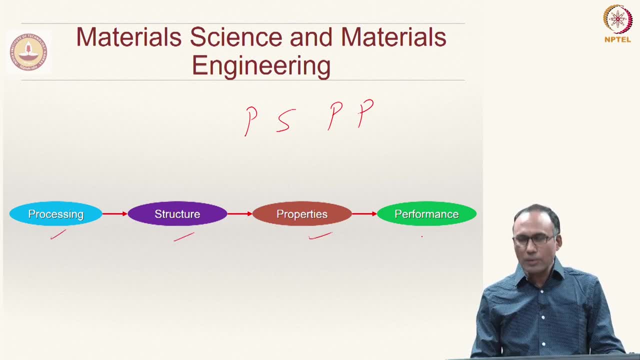 So here we see that the processing structure property performance. So the way that we should look at this line diagram is that we know, as we have discussed already, the properties of a given material depend on the underlying structure. So the different properties might depend on structure. 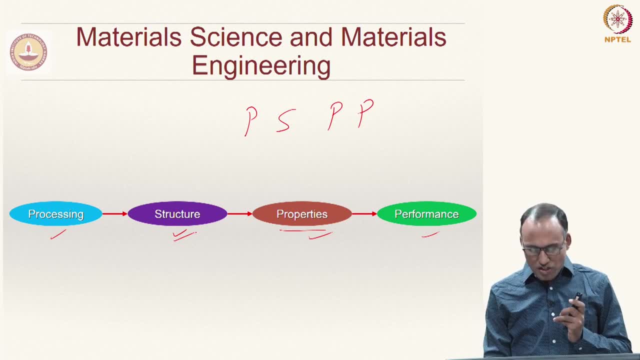 Structure at different length scales, but there is a clear correlation between the structure and properties And once you have a property and using a material of certain property, you can define what is going to be the performance of a component made of that particular material right. 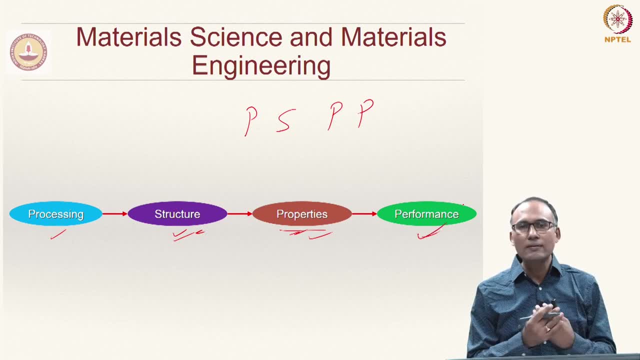 So the performance of a component that we are designing or using, out of using of a material, of a particular material, depends on its properties, right? So, for instance, if you are talking about design, So you are designing a shaft and you want to ensure that the shaft does not yield during 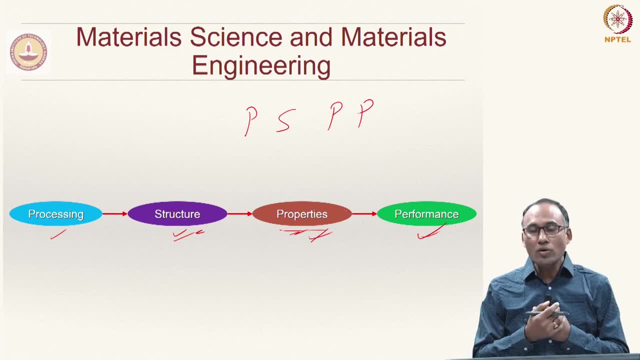 operation. that means that does not plastically deform. So the yield strength of the material is a property of the material. for instance, the shaft is of made of steel, then the yield strength of this steel is a property that is going to determine what is the performance. 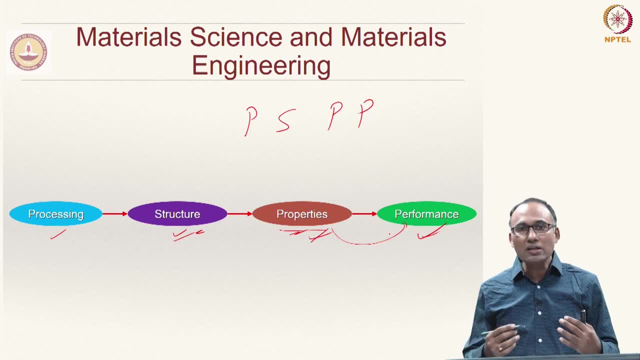 What do we mean by performance here? when we are applying a load, whether the material will yield or not under the applied loading scenario that is prevalent for that particular structure. So the properties, So the properties closely govern how the material, how the component that you are going. 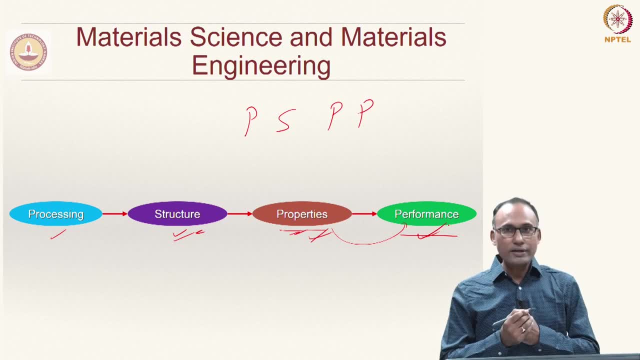 to design out of this material is going to perform all right. So where does processing come into picture? So we said, the structure is what is going to give rise to a properties, but how one would obtain structure, a given structure. So the processing route that one takes in order to develop a particular material determines. 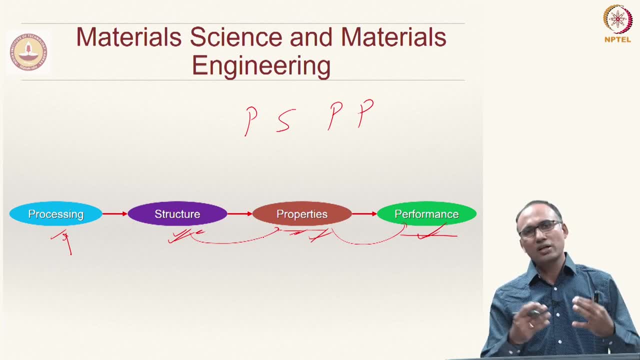 the structure that is going to be induced in the material. So the processing route that one takes in order to develop a particular material determines the structure that is going to be induced in the material. So the processing route that one takes in order to develop a particular material determines. 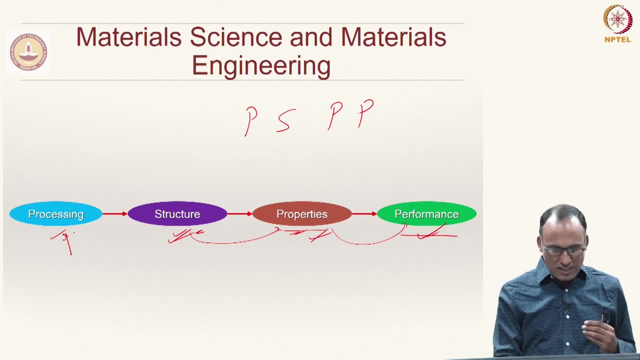 the structure that is going to be induced in the material right, Particularly at the atomic and higher length scales. So the processing is the key, which will give rise to a structure and that in turn gives certain properties that will determine the performance of the component. all right, 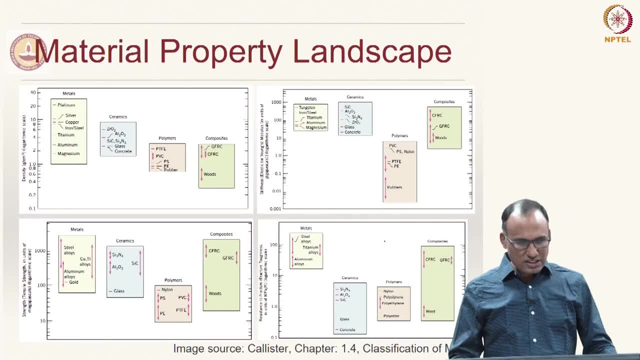 So, having discussed the fact that the properties are going to the one are the important aspect of the material which is going to govern the performance of the component. So this is the key, So that is the key, So that is the key. 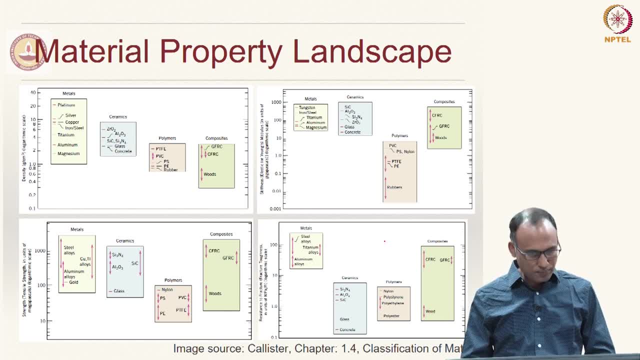 So here we are going to look at the material property landscape. here we are looking at four different properties. However, there are other properties which are of importance in general, but here in this class, we are going to look at these four important material. 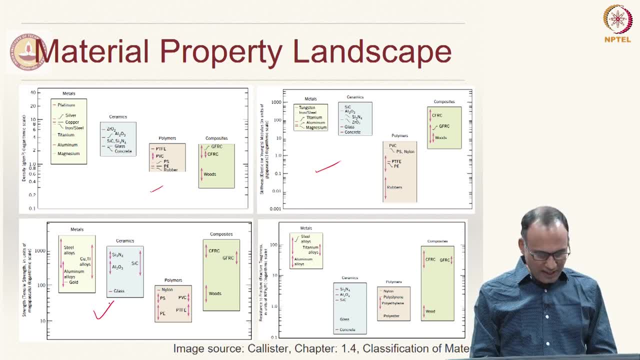 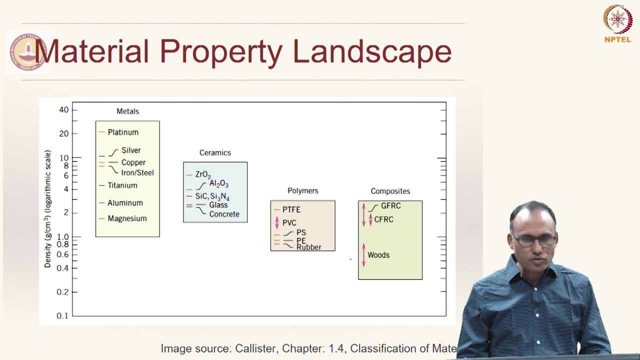 properties called density, elastic stiffness, strength, tensile strength and fracture toughness. So let us look at each and every one of them. So here we are showing density for different class of materials. So we have four different classes: metals, ceramics, polymers and composites. 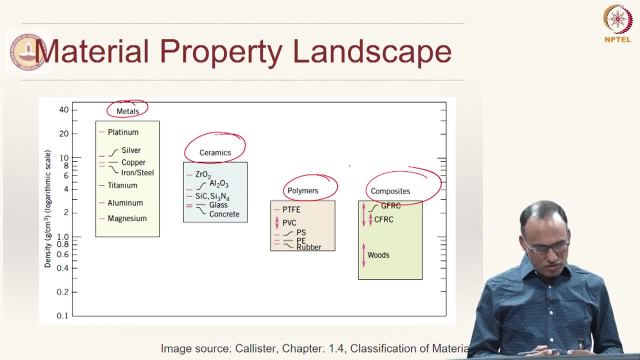 So we see that the metals seem to have a range of density. So that means different materials. if you are taking materials falling under the class of metals, the metals seem to show a large range of variation of density. There are materials which are extremely light. 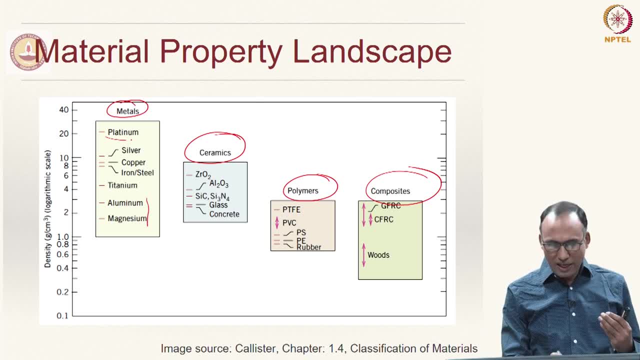 like aluminum and magnesium, but extremely heavy, like materials like platinum, silver, copper and so on. So, in general, the metals show a wide range of densities, but they are usually known to be heavy, heavy elements. And now let us look at the ceramics. we will see what are ceramics. 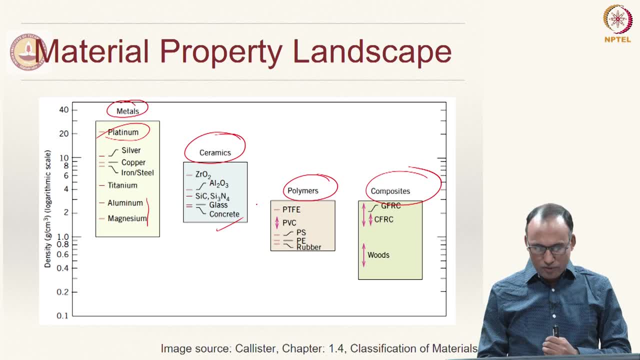 at in a couple of minutes. So ceramics actually show the densities which is within the range of these metals, but they are usually their highest density is usually lower than the highest density of metals, So they are relatively less dense compared to metals, and polymers are much less are known. 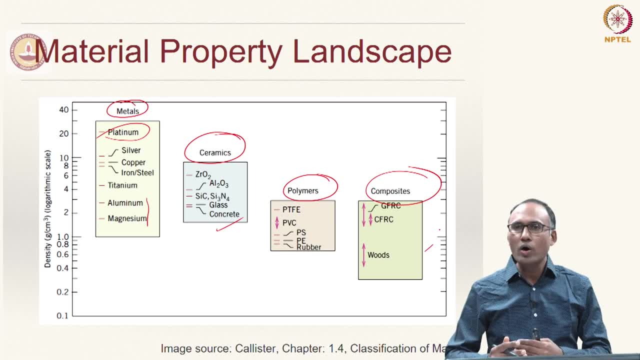 to be light and composites, again, can show a large variation again. but the composites will, as we have seen, as we can see here, also show a large range of densities, but still you can have these densities of these composites to be much less than the metals themselves. 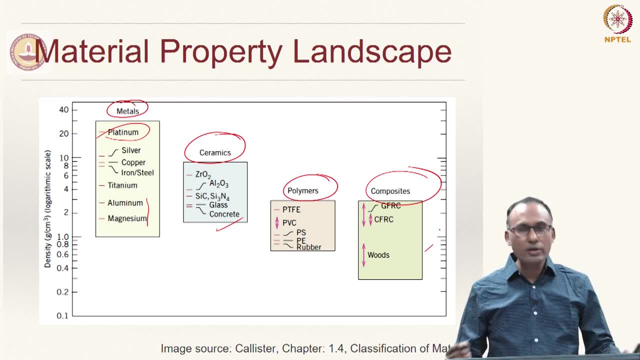 So if you are looking at the design of a particular composite, you can see that. the nice thing if you have drawn up again that there are so many active and upgraded bits of Din noods, and all right, So I can show you one. that is the arms. that is what I can do. you can see that in this. 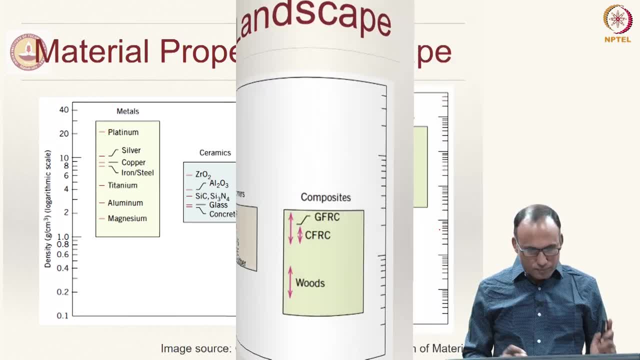 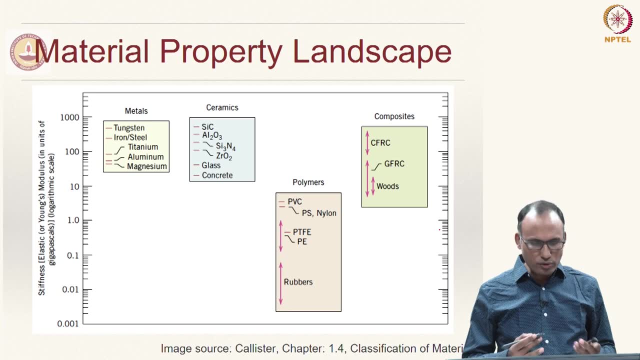 painting. I am firstly showing you that, the ARM ball of bond. you can see that I am noticing that it is very large size. So arm of bond that is very large basically, which will become like an arm. So they have the size in them, but just please note that only that size For these structures. 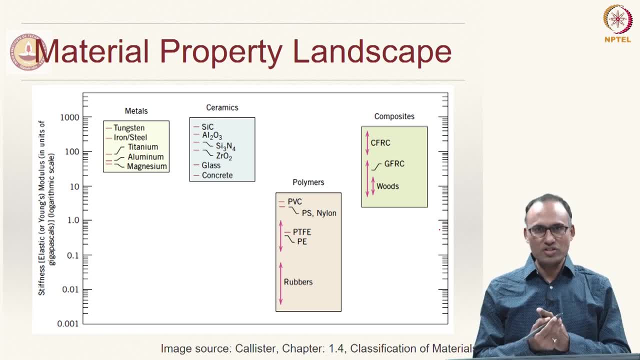 which you bring Peach pressure that match and is close to so the size is based on the lateral dies, the resistance to deformation, right. So if you, what is this elastic stiffness or angstrom modulus of elasticity if you have, if you remember your applied mechanics? 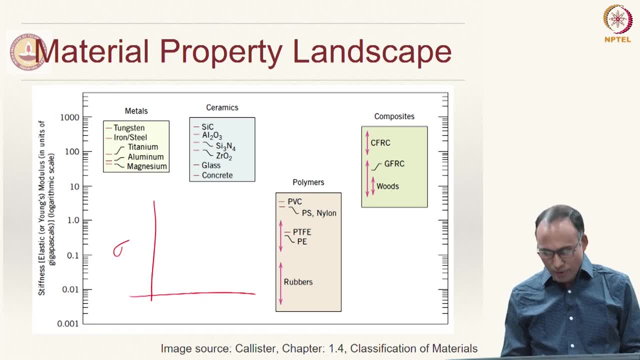 lab where you have done uniaxial tension test on a material, particularly probably you would have done on steel, Then you would have got the linear elastic part. this is the slope of this guy- is what is called elastic stiffness and that is what is shown here, right? 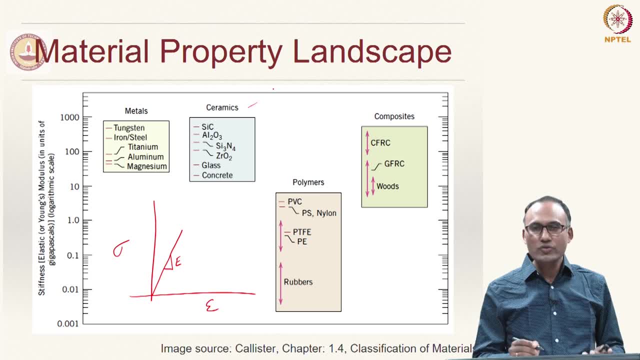 So here you can clearly see that the metals and ceramics show very high stiffness, while polymers show low stiffness, and of course you can have polymers of different kinds which are spanning from very low stiffness to a moderate stiffness. So for a metal- ceramics- 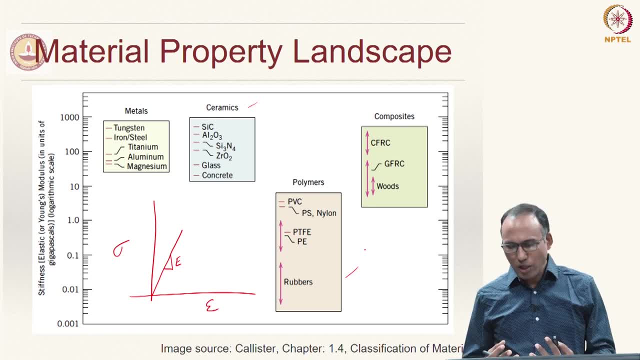 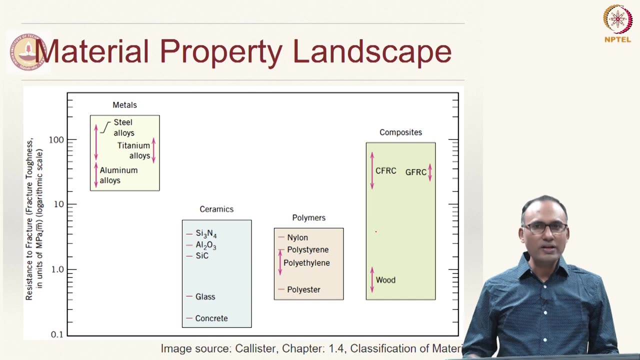 and are going to show very high stiffness values by polymers. and polymers show very low stiffness. that is probably one of the weakest points of polymers, and composites again can show moderate to high values of stiffness. And now the third property that we are looking at is the fracture toughness. So the fracture. 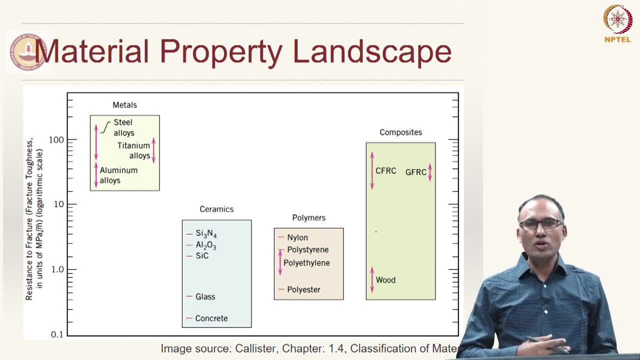 toughness is nothing but is the resistance for the crack propagation. or in other words, the toughness of the material is the ability of the material to absorb energy before actually going to fracture. So the more amount of energy that it can absorb is means that it has more fracture toughness. Again, metals win here. they have extremely high fracture. 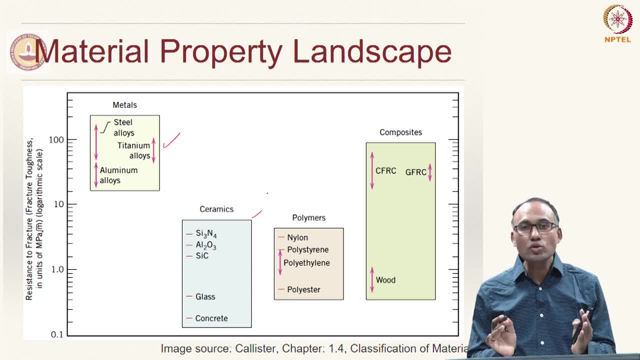 toughness. Compared to ceramics, ceramics are not known to be tough, right, they are highly brittle and hence, if they fail, they fail suddenly, while metals will give you some indication that they are actually going to fail. So ceramics are known to be known to be materials. 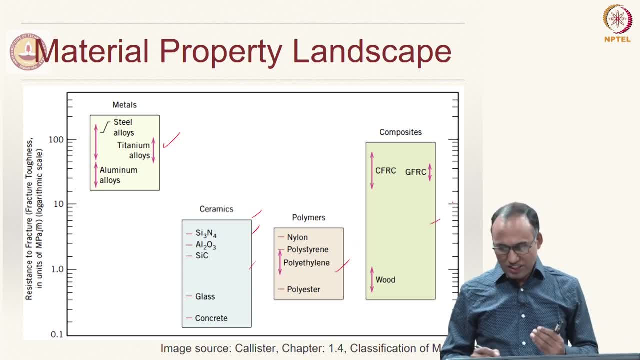 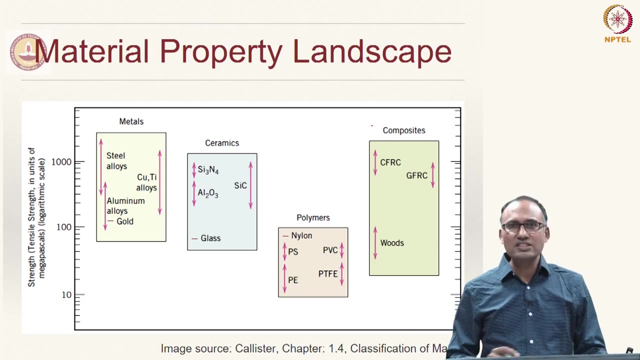 with low fracture toughness, similarly polymers, but again composites. here have again a range, So they go from very low fracture toughness to almost Similar fracture toughness as metals. And last property that we are looking at is a tensile strength. So tensile strength means 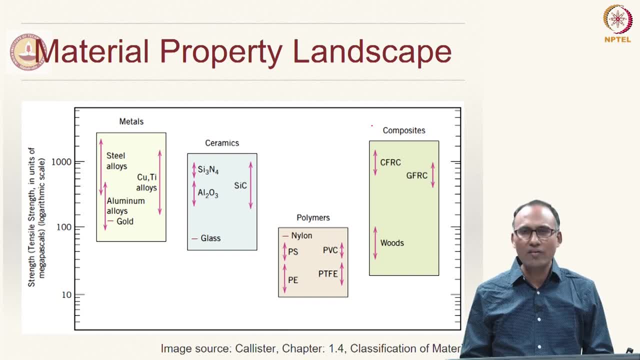 basically ultimate tensile strength of the material that we have already. you probably have already measured for steel in your applied mechanics lab. Here you can see that the tensile strength of metals again is higher and ceramics also have similar or sometimes more tensile strength. 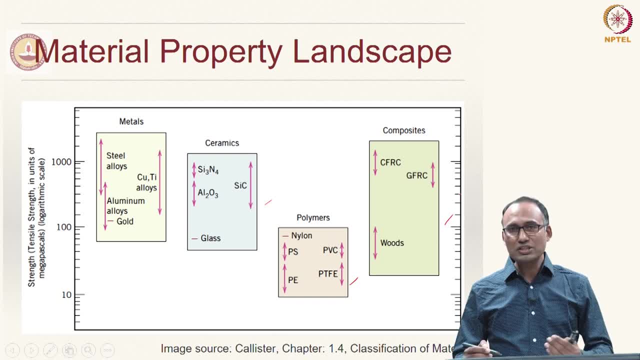 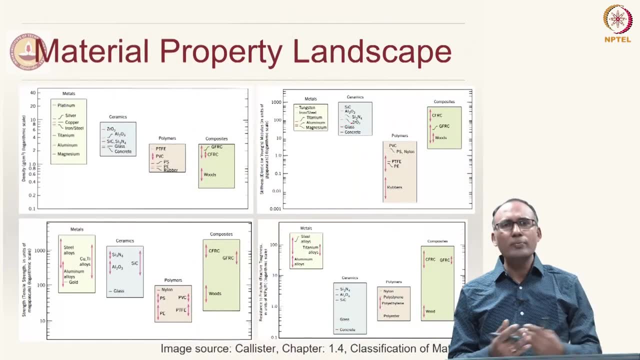 So they again have a low tensile strength and composites again have a range very low value to very high values, right, So this is how the different kinds of materials showed properties, exhibit properties, as we have seen here and by looking at this material property. 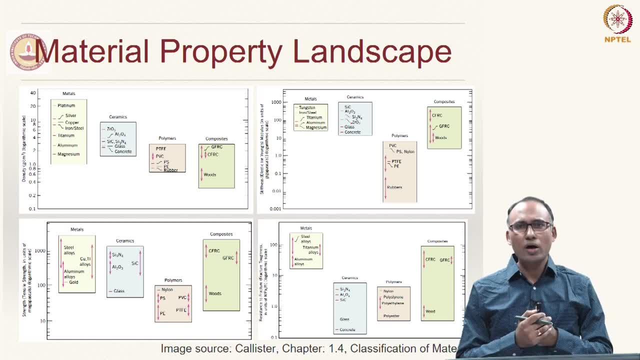 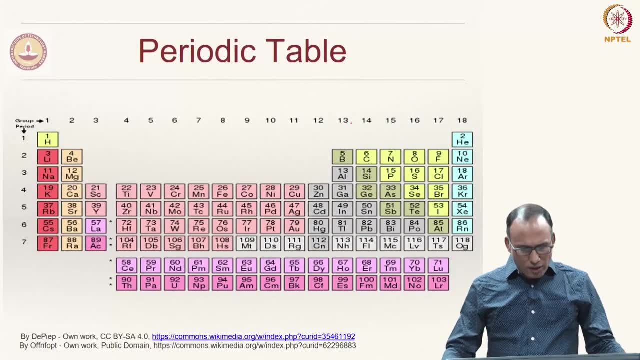 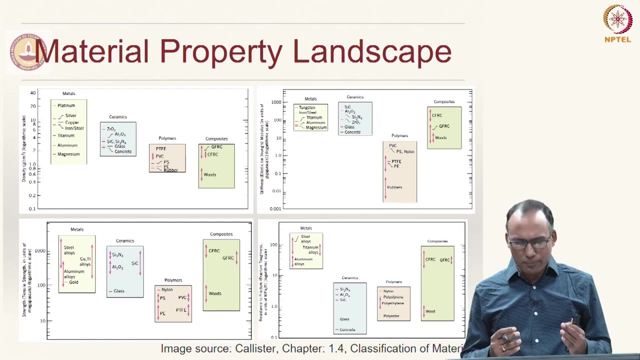 landscape, one can make an informed decision on what will, on the choice of the material for a specific application. alright, So let us look at. So you, you have seen that in the previous graph, the metals, and of course in this course we will be focusing only on the study of metals in particular. and So here we can see that. 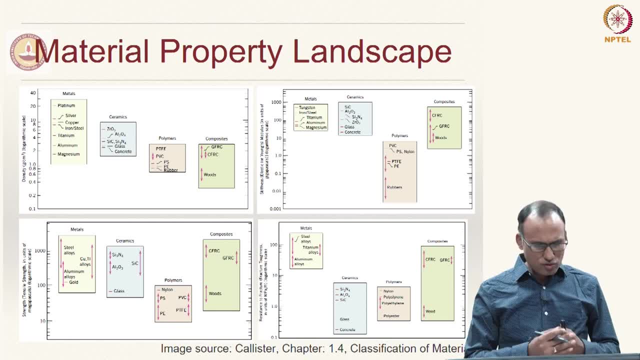 metals seems to have all these properties at the higher range. So, including the density, that is probably one of the downsides of metals, because they are heavier, but otherwise they show very good strength, very good stiffness and very good fracture toughness. alright, 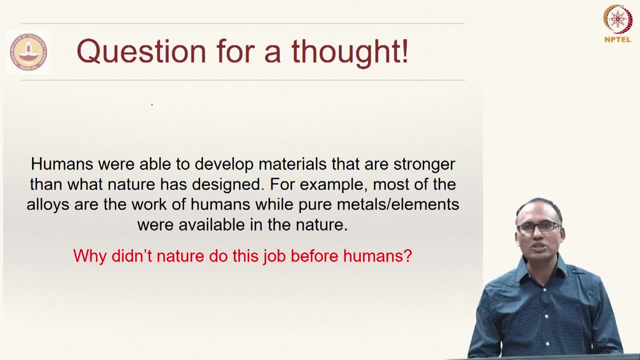 So that is the work of humans, while pure metals or elements were available already in the nature. So if humans could do it, why did not nature do this job of making stronger elements, stronger materials or alloys that humans could make? Think about it and try. 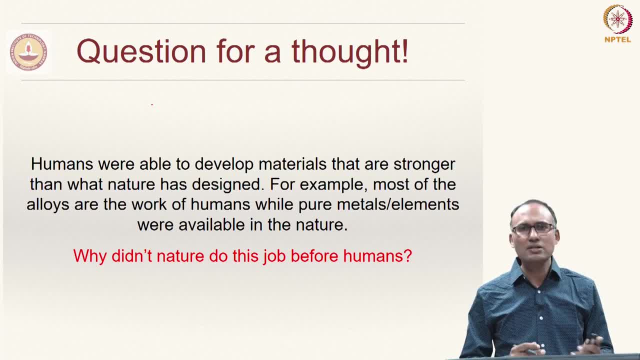 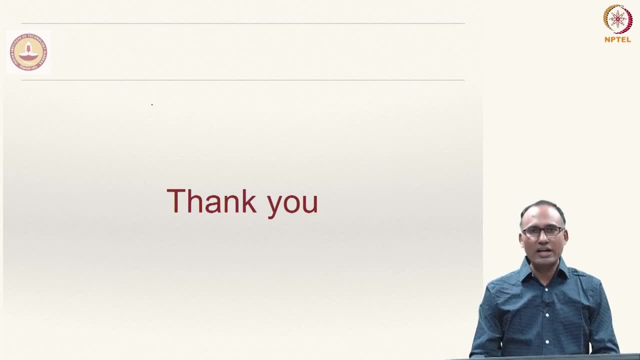 to find an answer, and we hope to find this answer for this question probably during the during this course. So with that, thank you for your attention.